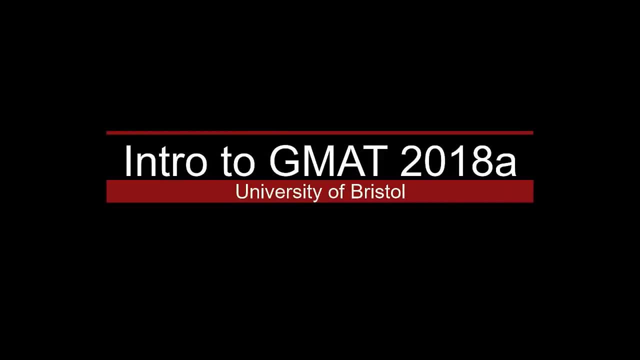 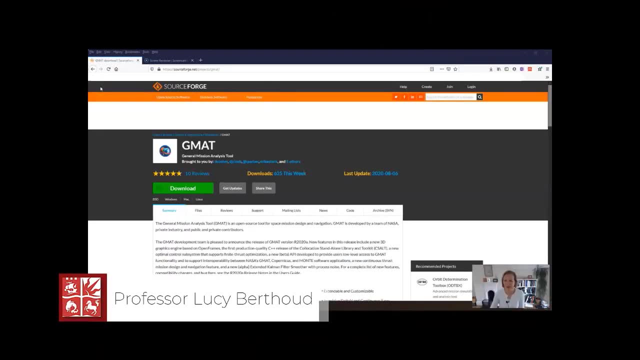 Hi, this is Lucy Bertu from the University of Bristol doing Space Systems Engineering and an introduction to GMAT or General Mission Analysis Tool. It's a great open source tool for space mission design and navigation and it was developed by a team of NASA, private industry and public and private contributors. 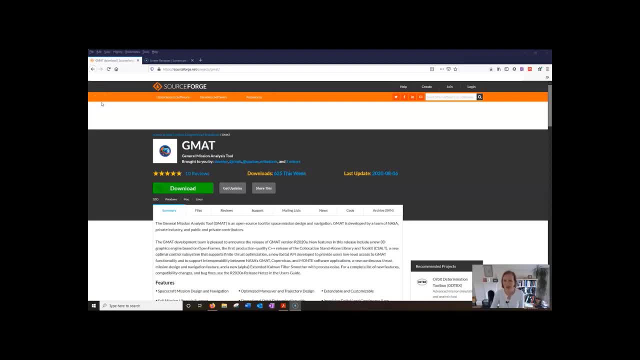 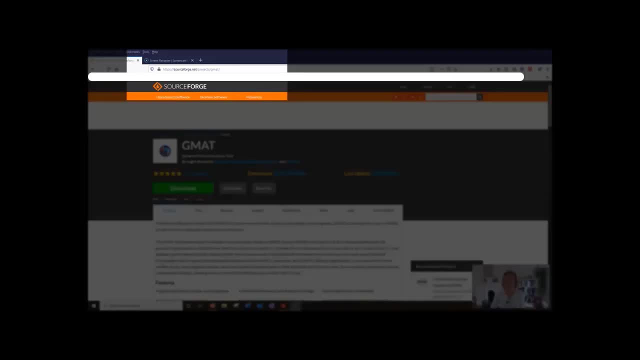 What we're going to have a quick look at in this video is how to start off and just the basic menu structure. To find GMAT, first of all go to sourceforgenet and projects and GMAT. You can just Google that. 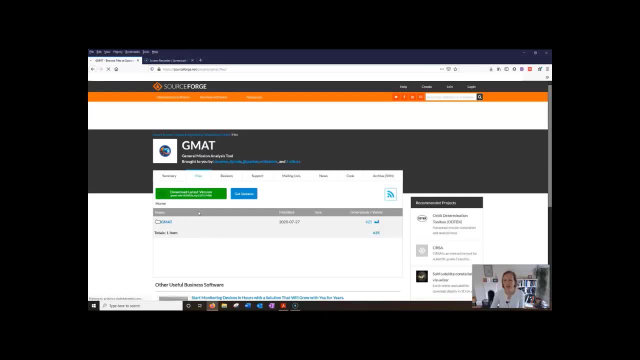 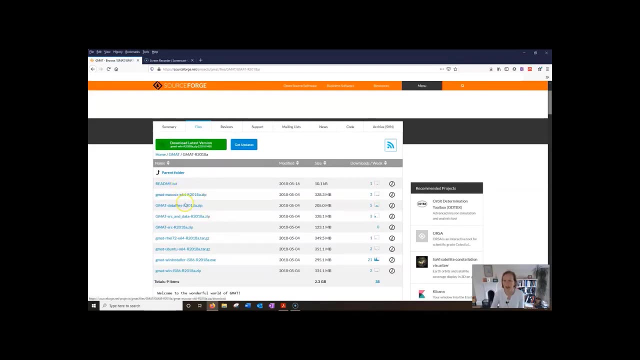 And then, if you go to files and then GMAT, then you should be able to see all the different versions. We're going to choose 2018 because that's the version that's compatible with the ones on Google. You can see here all the different versions. Here's the Mac version. 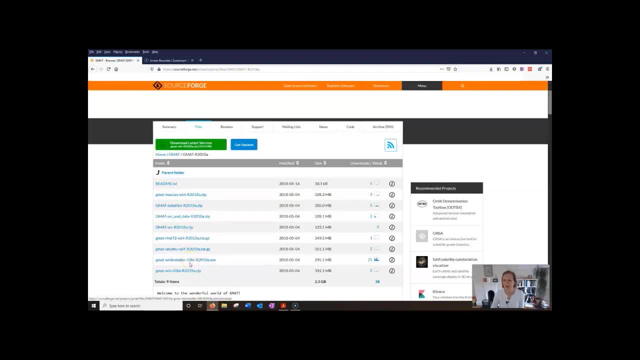 There's Red Hat and Ubuntu. for Linux. There's a Windows installer and there's a binary bundle of Windows as well, So you can just install whichever one is suitable for your machine. Once you've got it installed, and make sure it's all in the same file folder to conserve the structure of the folders. 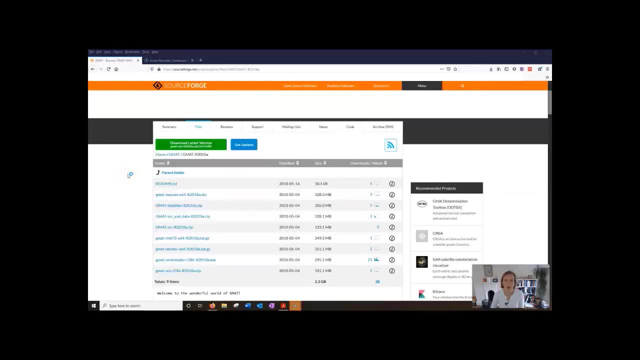 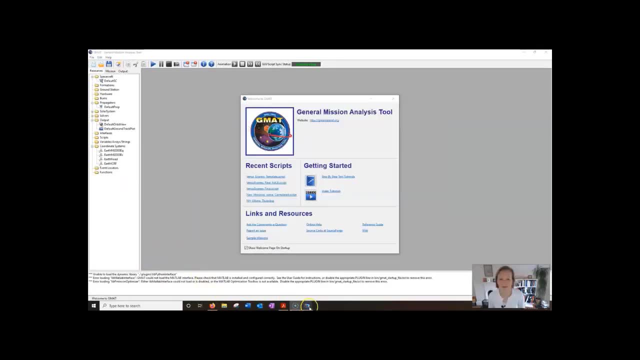 then you're just going to click on the app Or otherwise go to the exe file to run. it Takes a little while and then it's going to come up like this: Here's the welcome screen and you can see on it there's some quite a few helpful, helpful things here. 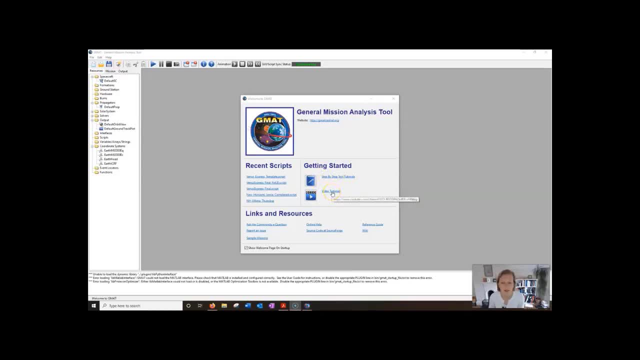 There's some step by step text tutorials and then there's some video tutorials. It has your most recent scripts up and then there's a whole bunch of links and resources which are really useful. There's the source code. There's a reference guide That's like a user guide. 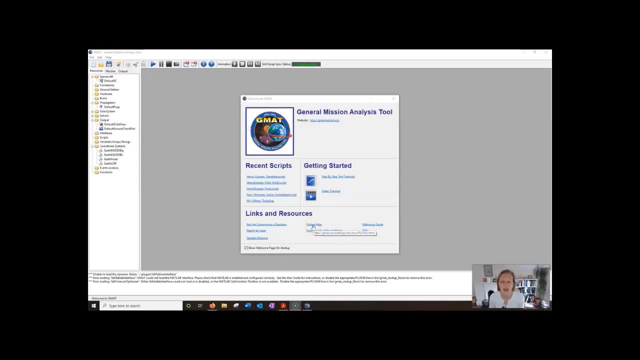 There's the wiki, There's also an online version of the user guide, Some sample missions, which are really nice if you want to expand your learning and look at a few other things, And there's also like a discussion forum there and you can report an issue. 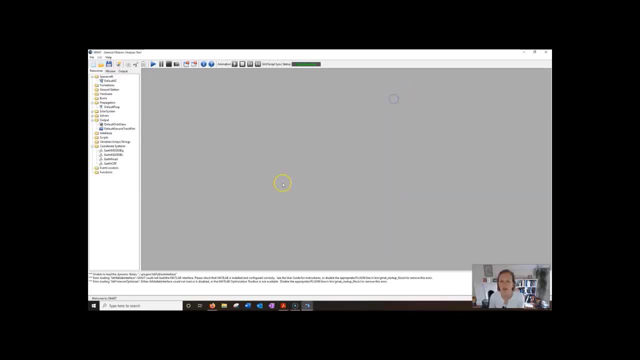 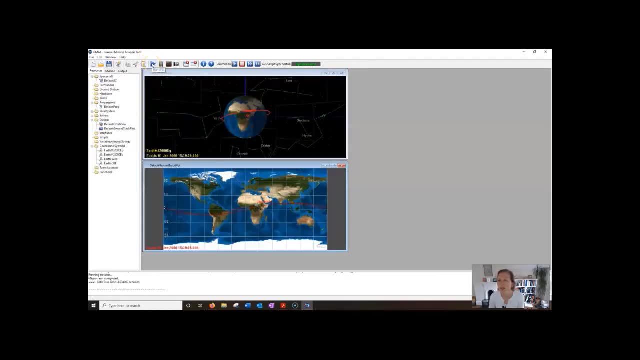 So all of those useful, But you may want to get rid of this file, just for the starters. So what we're going to do, we're just going to press. I just press the run button there, That's this one here, And it's going to run the default mission. 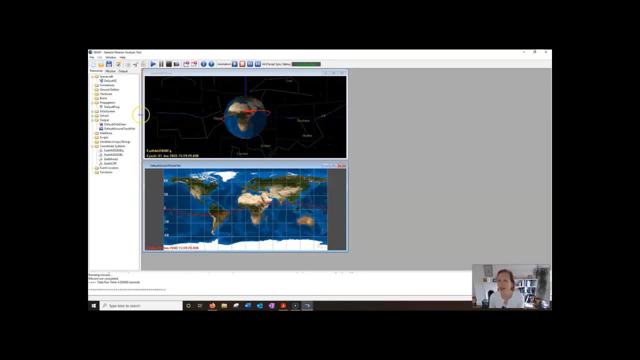 This is just something to get you started And you can see here we've got three tabs. We've got a tab which is called resources- We can have a look at these in a minute- One called mission and one called outputs. OK, at the bottom we have some messages from GMAT, which is useful. 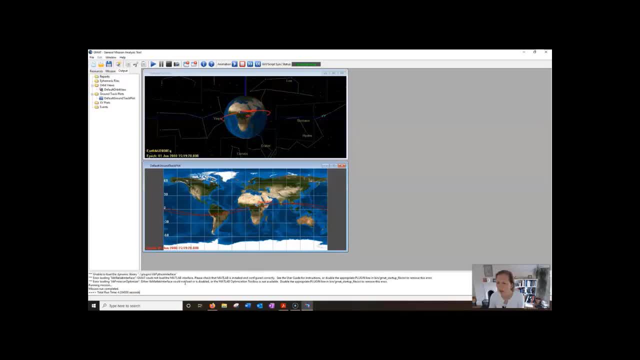 And it'll often say mission run complete. If I scroll back, you'll see that there's some little error messages: Unable to load the dynamic library, error loading fmincon and so on. Don't worry about those, Those are just compatibility things. 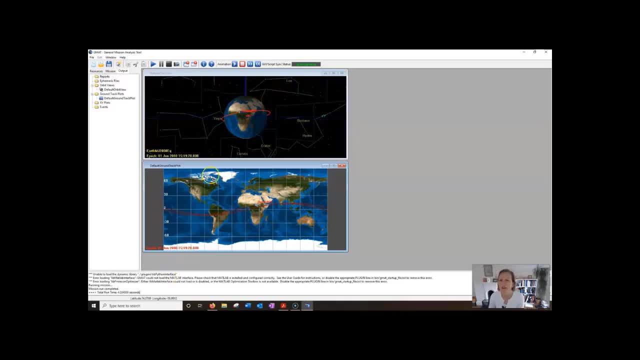 And it's not a problem for what we're using it for. OK, so on this main screen you can see an orbit view and you can also see a ground track view, And if I go to the play button for start animation- this blue one here- then you can see my, my little satellite moving there. 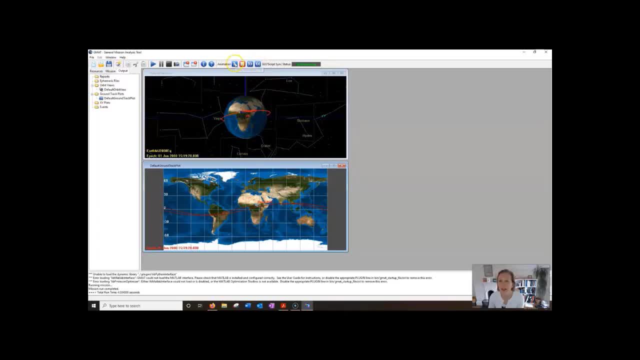 So I can slow down the animation a bit And play it a bit once again, Or I can speed it up here. I can stop the animation. That's also quite useful if you're halfway through and you've realized already what you want to fix. 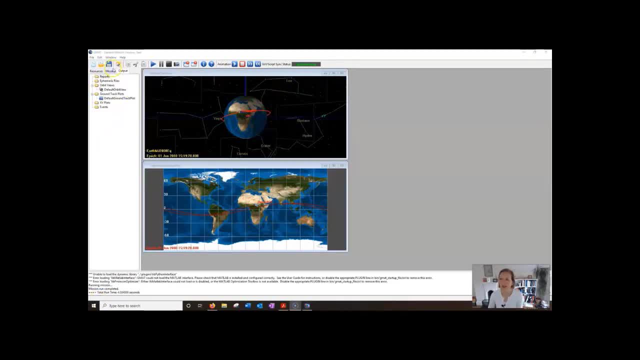 So that's also useful If you're going to save files. you can have the usual sort of open a recent save and save as That's all under file. You can look at various different versions of the windows. You can tile them horizontally. 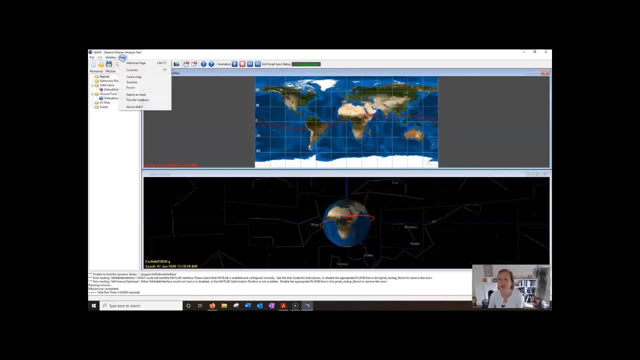 And so on. So you can just have fun with that. And then here we have once again some links for the help to the various different resources. I would highly recommend saving your mission here, or file save regularly, Just because just occasionally, GMAT does crash and it's possible to lose everything that you've worked on. 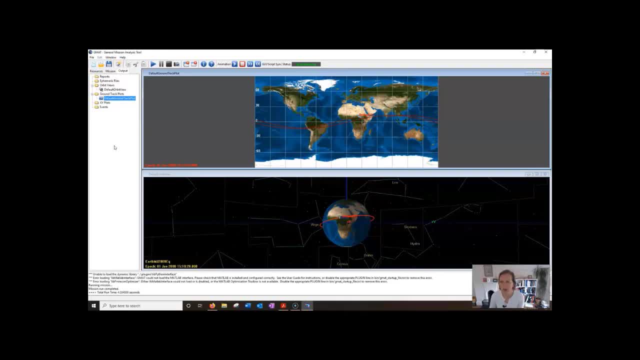 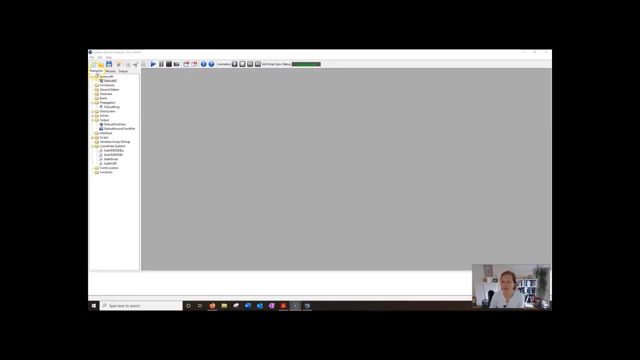 So please save regularly if you want to save yourself some GMAT tiers. Let's go first of all to the resources tab. The resources tab is where all the GMAT resources are organized into logical groups And you can either add or edit or rename them or even delete them if you want. 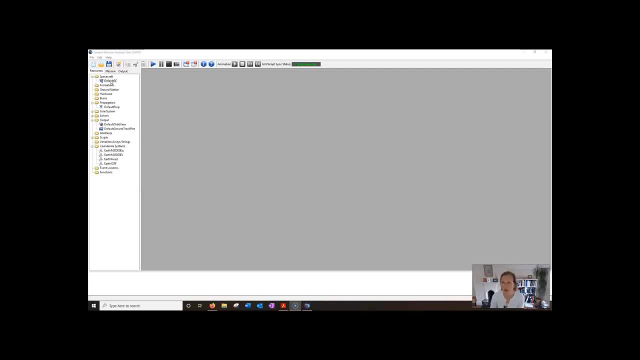 So you can edit it either directly in the GUI, like I'm doing now. So, for instance, we can go into the default spacecraft. We can change the Epoch format to something a bit more familiar. That'll give us UTC, Universal Time, Gregorian. 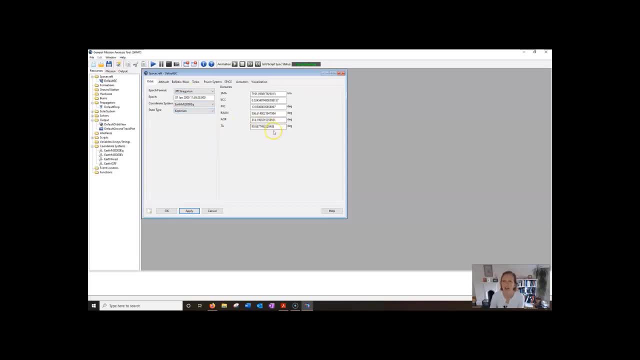 And then we can use maybe Keplerian elements, for example, So we can edit this in the GUI, or we can go to scripting. This is slightly more advanced, But, for example, I've got a script here and I can double click on the scripting and I can go into this. 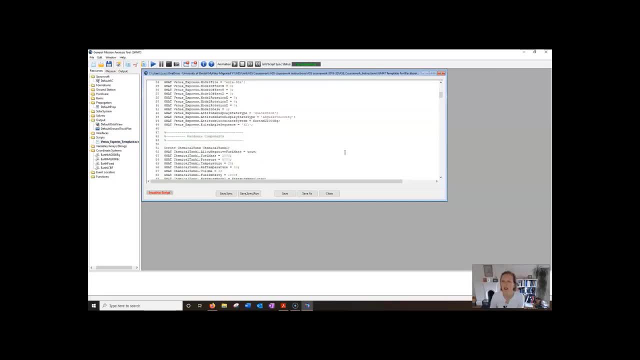 This scripting is kind of MATLAB based, So if you're familiar with MATLAB then you'll see it's very nicely set up. You can see all the force models and you can see. you can either upload or just edit directly into the script there. 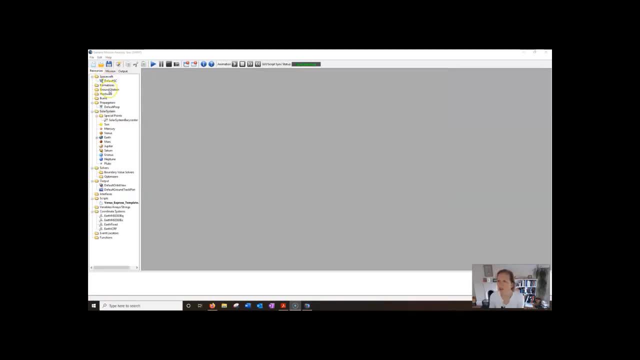 So in the resources tree you can add in spacecraft, you can add in ground stations, you can add in fuel tanks to the hardware, different types of burns, different types of propagators. You can see here I've expanded the solar system. 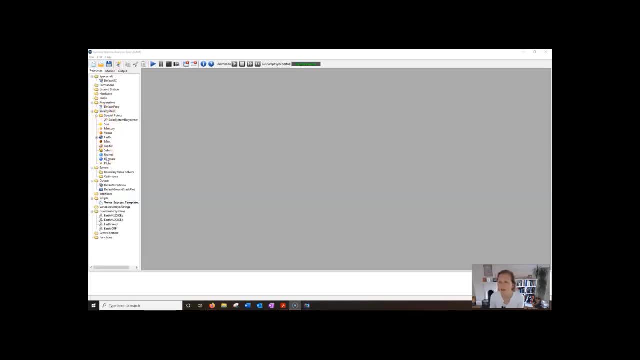 So we've got all the planets. that are all in there, But you can add in moons or asteroids, different solvers and optimizers, different types of output. You've seen the orbit view in the ground track plot and there's various different versions of those. 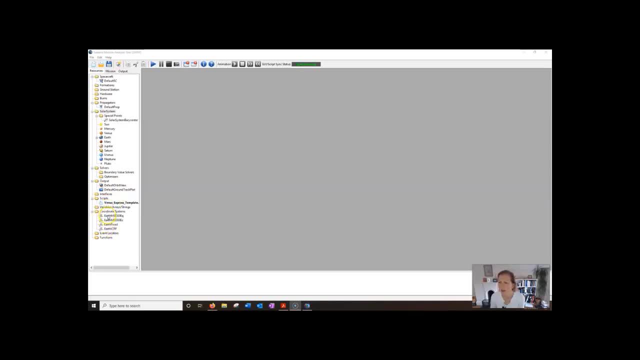 You've seen the scripts. These are the different reference systems which can be used for the orbit view, And that's useful too. The mission tree or mission tab, is in this part here, And this is a kind of ordered hierarchical display of your script commands for the mission sequence.